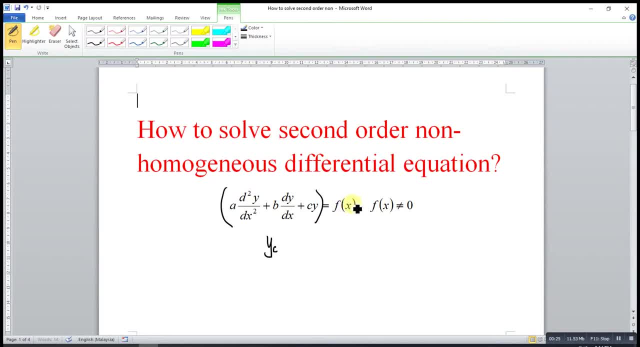 After that we find the particular integral for this non-zero function and we write as yp. Then the general solution is y equal to yc plus yp. Let's move to an example. So for this example, as we can see, the associated homogenous function is this, and then the non-zero function is 3.. 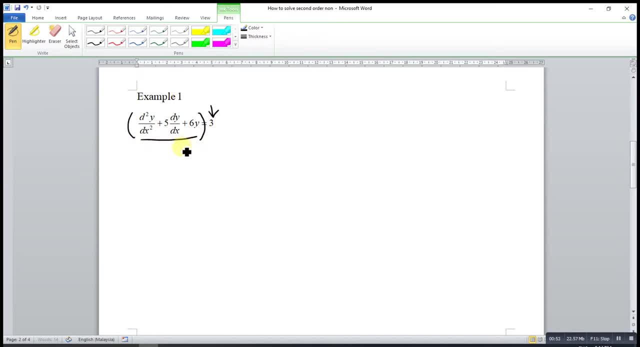 So what we have to do first is convert this homogenous equation to a quadratic function. So with the second order So m squared, we just introduce any unknown here. then plus we have a coefficient of 5, then we write 5, then this is first order, so m to the power of 1, then plus 6, then equal to 0.. 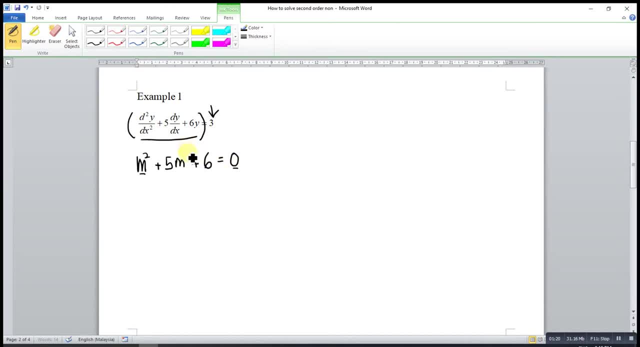 Remember we have to write 0 here is because of. this is homogenous function. Okay, after that we can factorize: Plus 3 equal to 0. So means that m equal to negative 2 or negative 3.. So means that our complementary function should be equal to a- e to the power of negative 2x, plus b- e to the power of negative 3x. 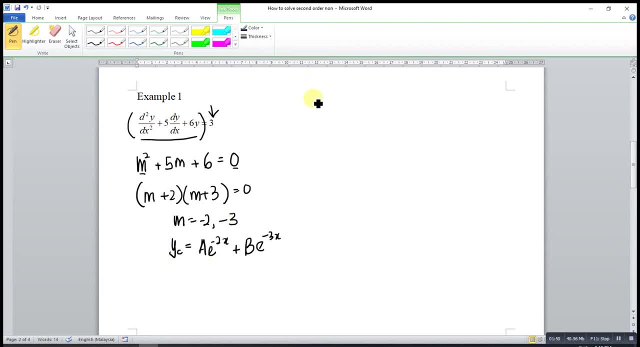 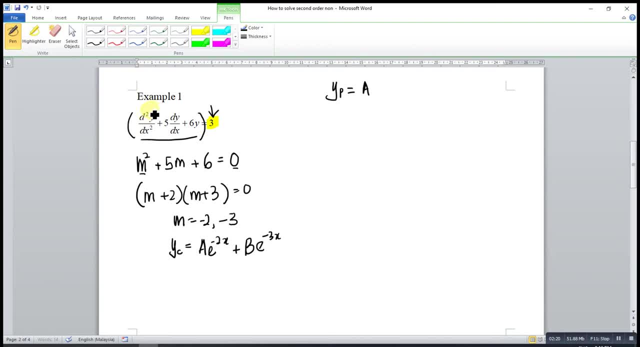 equation here. as we can see, here we have derivative up to second order, so it means that we have to differentiate for two times. so we differentiate for the first time equal to zero, since this is constant. differentiate a constant, we have zero. then differentiate for the second time, we get. 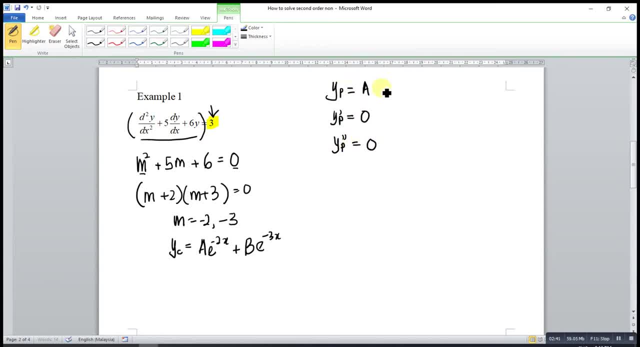 another zero, then after that what we have to do here is we substitute all this into this equation. so second derivative is zero. so zero plus five times the first derivative, zero plus six times the first derivative, a equal to three. so zero, nothing, we just cancel. so means that 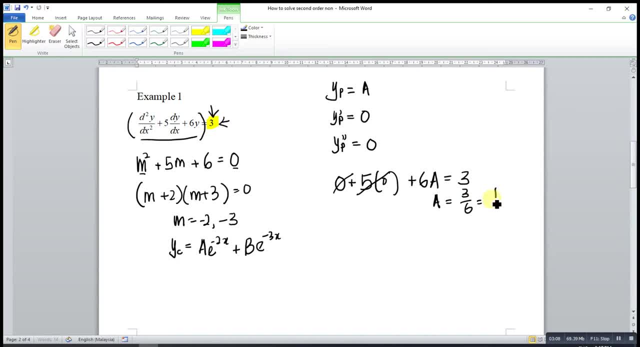 a equal to three over six, which is one over two. so means that our particular integral equal to one over two. then we have y equal to yc plus yp. so means that our general solution for this differential equation is: a: e negative two x plus b, e negative, three x plus one over two. then we're done. 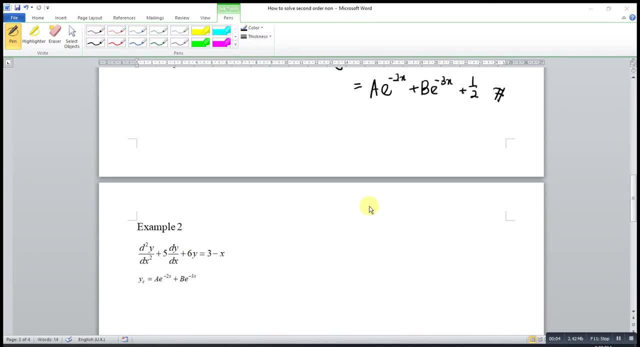 let's move to the second example. so we remain the homogeneous part and we change the non-zero function to and we change the non-zero function to and we change the non-zero function to a linear function. so for this linear function we just let y p equal to. this is linear. so a x plus b. 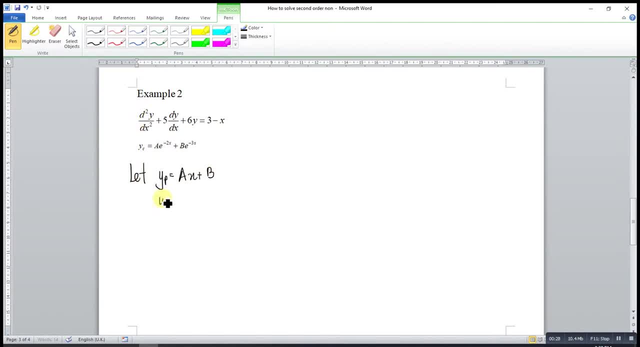 so, as we can see, second order. so means that we still have to differentiate for two times. so when we differentiate for the first time, ax, we have a, then plus a constant. where we differentiate zero, so we differentiate for the second time, we have zero. then we substitute all this. 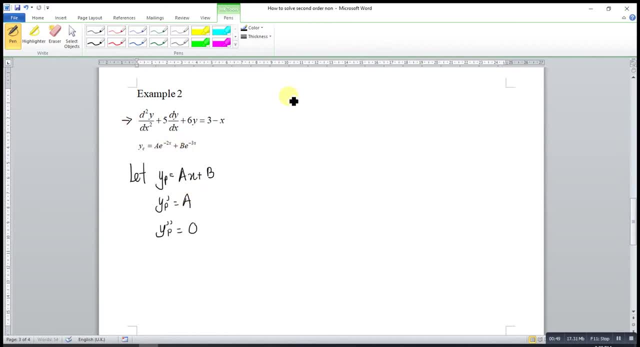 to the equation. so second order is 0 plus 5 times the first order, a, then plus 6 times the y, so a x plus b, that is equal to 3 minus x. then we group according to the unknown. so what we have here is 5 a plus 6 times ax, so 6 a x. then 6 times b, we have 6 b. 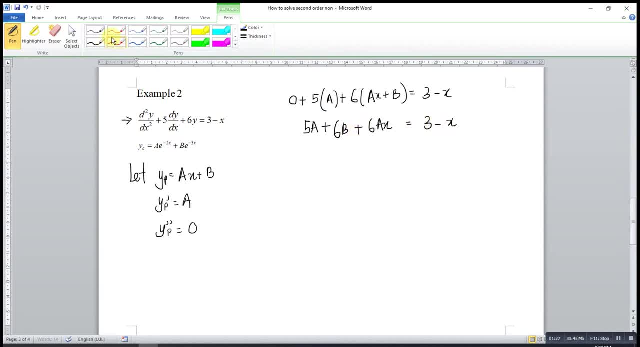 then equal to 3 minus x. okay, as we can see, the coefficient of x is negative 1, so negative 1 should be equal to 6, a, so it means that a equal to negative 1.. this indicates that a equal to 1 over 6 with a negative. 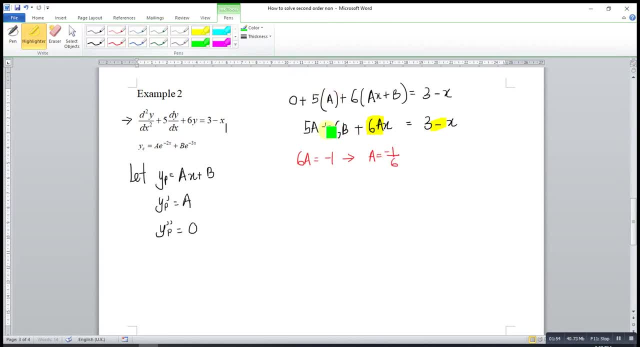 okay. after that, we find the remaining part okay, for the constant is equal to 3, so means that 5 a plus 6 b equal to 3.. this indicates that, okay, from here we have 2 x plus 6 times a plus 6 b. 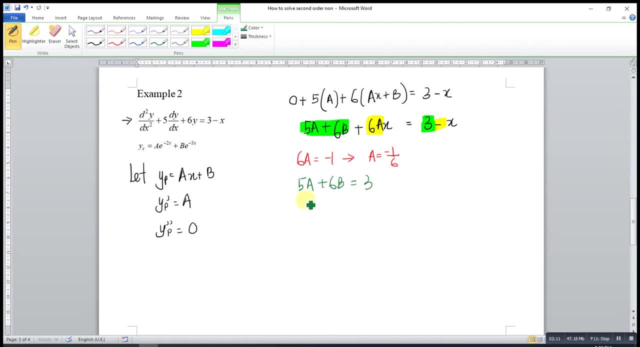 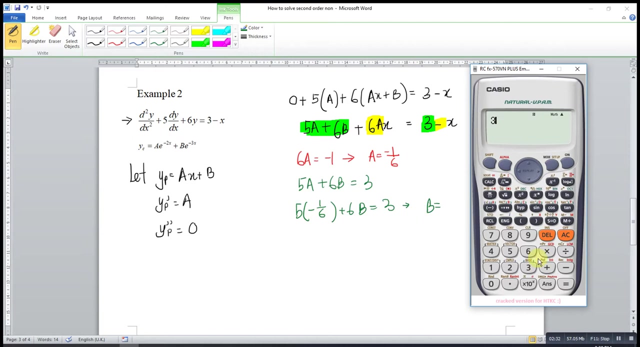 we have two unknowns, but a already found. so we substitute 5 times negative 1 over 6 plus 6 b equal to 3.. so this indicates that b equal to okay, we can use calculator. so from here three minus spring over becomes plus 5 over 6.. 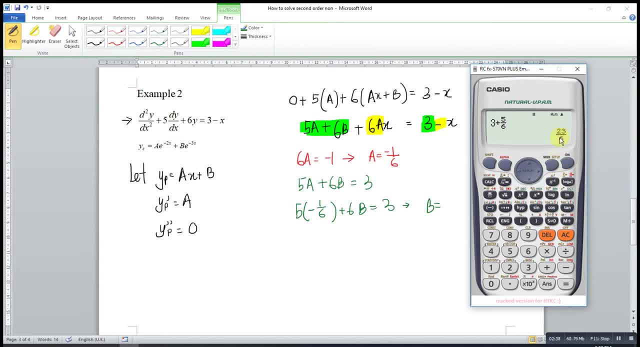 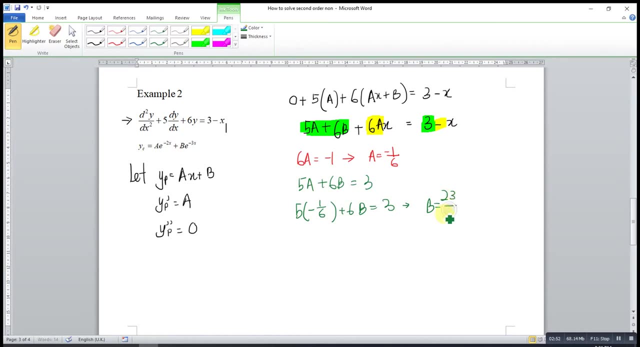 6. then we have 23 over 6, then 6b equal to this one, so 6 move over, become divide. then we have 23 over 36, so b equal to 23 over 36. so it means that our particular integral equal to. 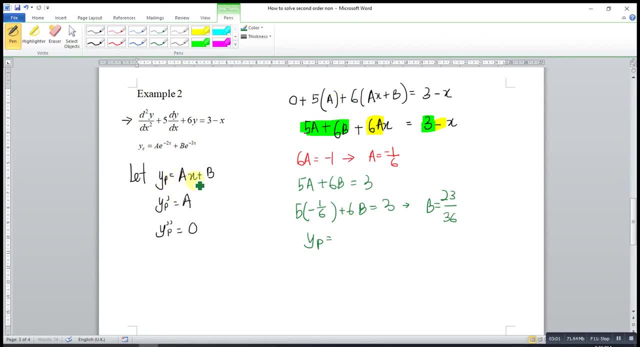 ax plus b. a equal to negative 1 over 6. x then plus b, b is 23 over 36. okay then we from our tankers solution: y equal to y, c plus y, p, which is equal to a a times e to the power of negative. 2x plus b. e to the power negative. 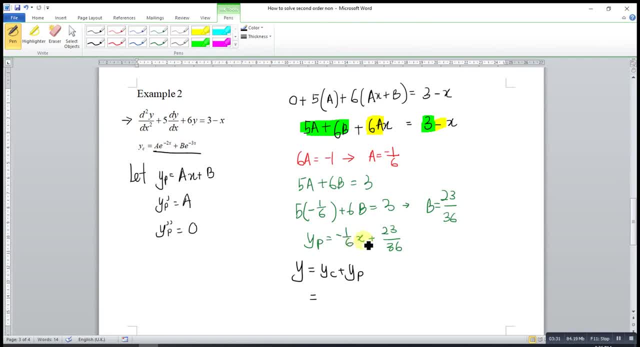 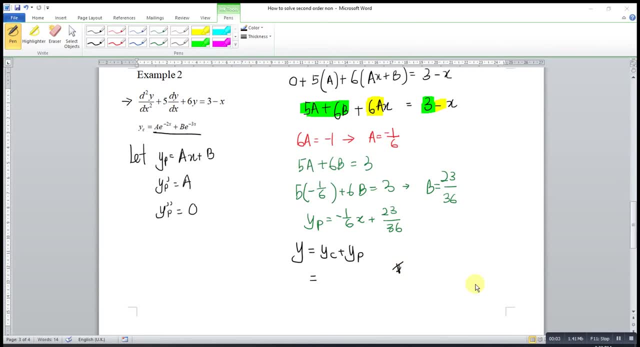 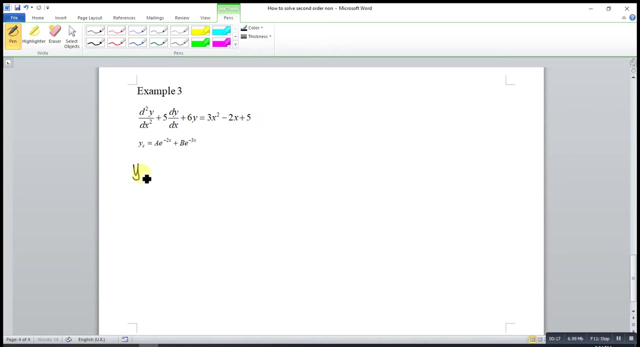 3x, then we have minus 1 over 6x, plus 23 over 36. okay, the last example for today. I remain the left side, but I change the right side to a quadratic function. yeah, so means that what we have to do here is our particular integral should be a. 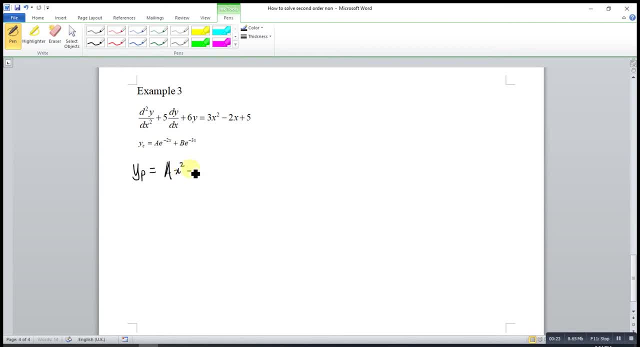 quadratic function. so ax squared my plus B, x plus C. so what we have to do also differentiate for two times. so when we differentiate the first time, we have 2 ax plus B. then differentiate again, we obtain 2A. then we substitute into this equation and we have 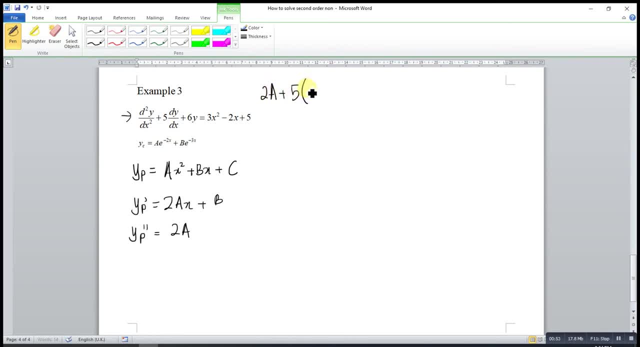 plus 5 times first order. so 2ax plus b, then plus 6ax square plus bx plus c, and this supposed to be equal to 3x square minus 2x plus 5. okay, then we according to the degree of x, so first we find the second degree. so for the second degree here, so means that we have: 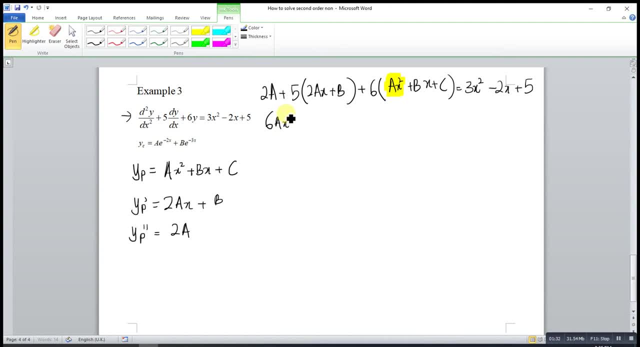 6ax square. okay, this part done. then we go to the x. okay, so this one, no x, this one we have. so we plus 5 times 2, so 10 a x, then plus 6b x, okay, and then we go to the constant part, so plus 2a plus 5b, plus 6c. 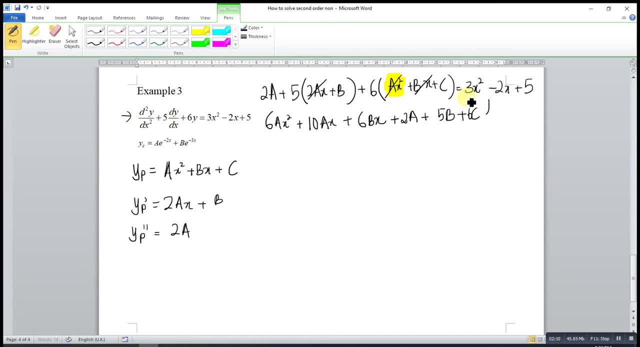 okay, and this is equal to this. okay, then we compare the coefficient. so we compare x square first. so x square, we have 3, since we have only one unknown so we compare x square. so we said 6a equal to 3. this indicates that a equal to 3 over 6, which is 1 over 2, okay, 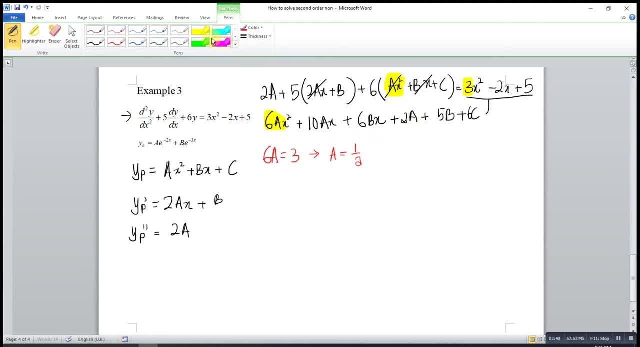 then we compare. okay, we won't take the constant part first, because constant, we have 3 unknowns. so then we see also, you see 1 minus 4a, a Something like this one. you can continue going until all we have to do is here, we go to the next stage, we show you what time number. 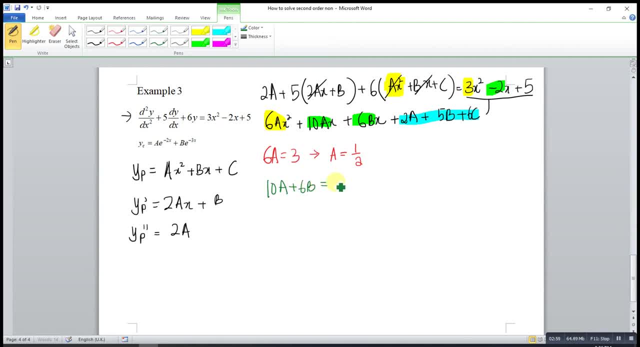 to what time NFOf is equals to, and this will be equal to negative two. so this is what we will buy to get minus three, and that will give us the net cost A for us class high model. so what we are going to do is take this to get the V first. so what is the nothing, of the non-none circle, and then 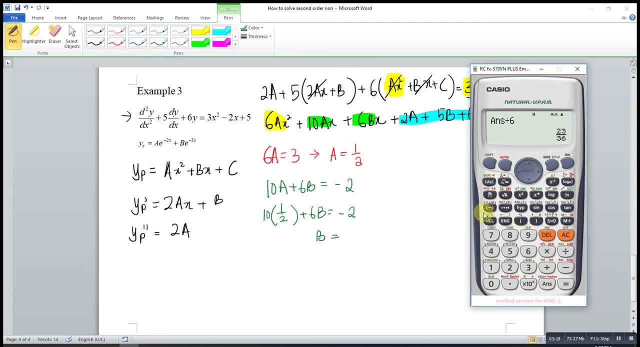 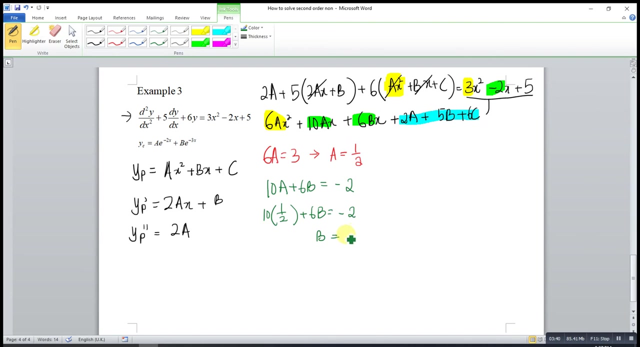 we are going to make aiş. we group them. and now let me cricket in the same group. now let's negative: 2, 10 over 2 is 5. positive 5 bring over, become negative, so minus 5, then we have negative 7. then times 6 times 6 here move over, become divide, so we have negative 7 over 6, 7 over 6. 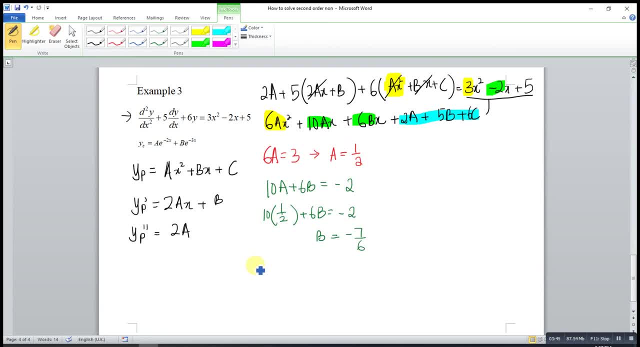 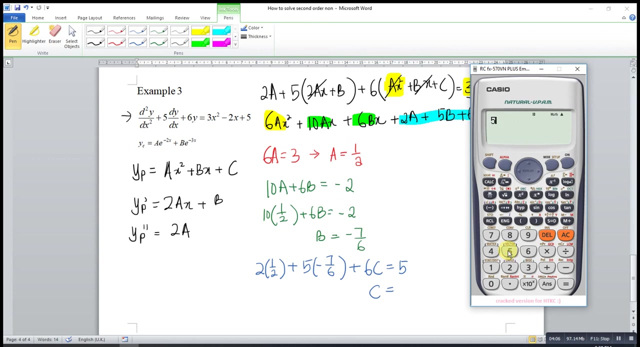 okay, now we do the remaining part. so 2a is 1 over 2 plus 5b is negative 7 over 6 plus 6c. equal to constant is 5. so c is equal to 5 minus 2 over 2. this one. 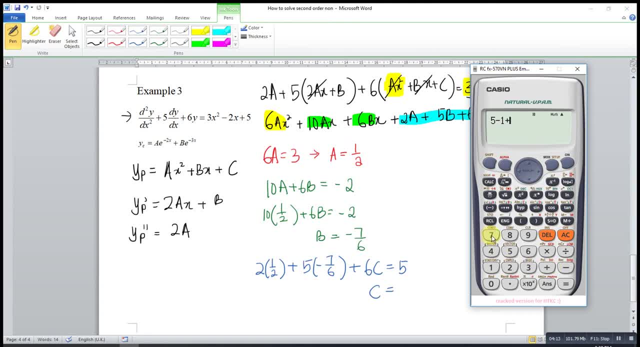 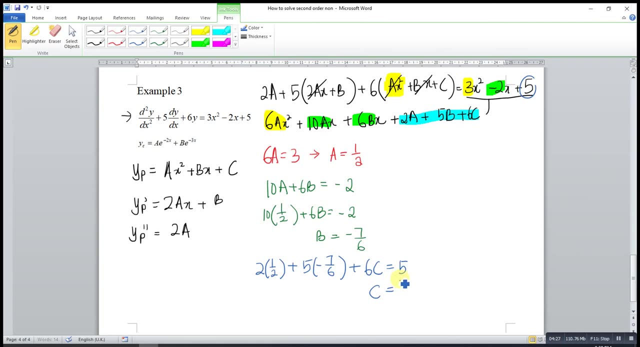 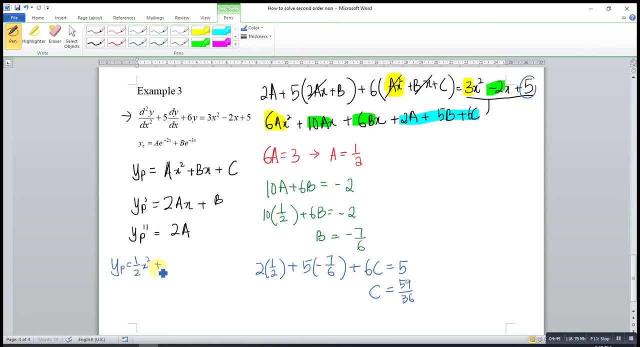 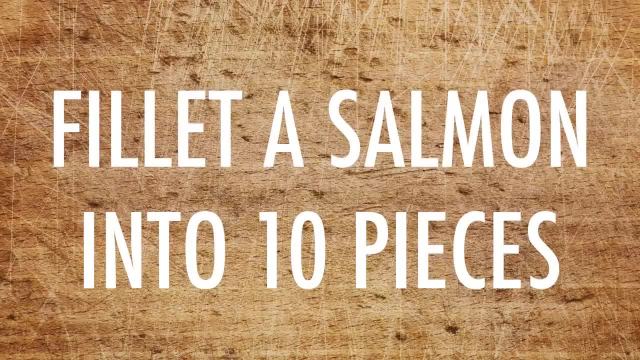 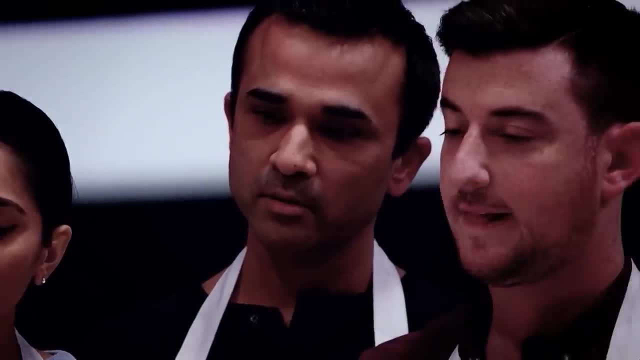 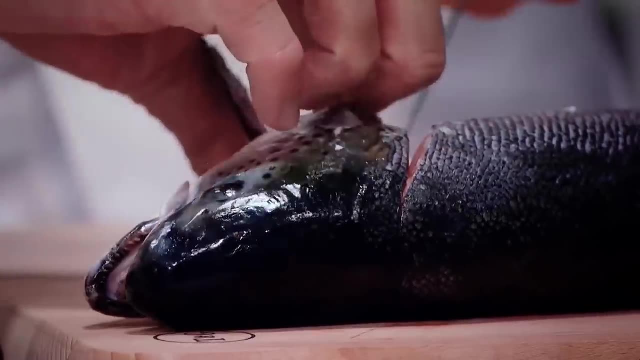 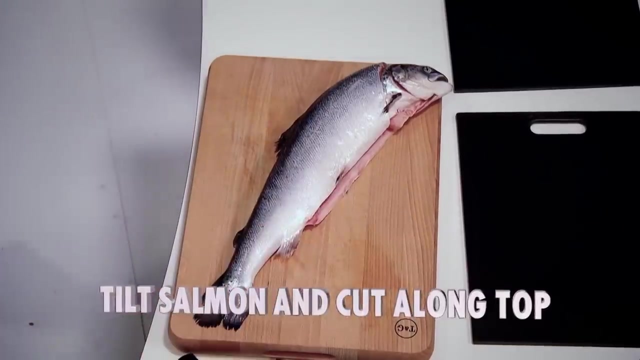 Finishing the salmon, make sure the scales are removed. Super sharp knife. Let the knife do the work. First off, knife: Look at the gills. Lift up the gills, slice, feel the bone halfway through and come down throughout. Turn the salmon around, tilt it. Once you tilt it, okay it'll help. knife. 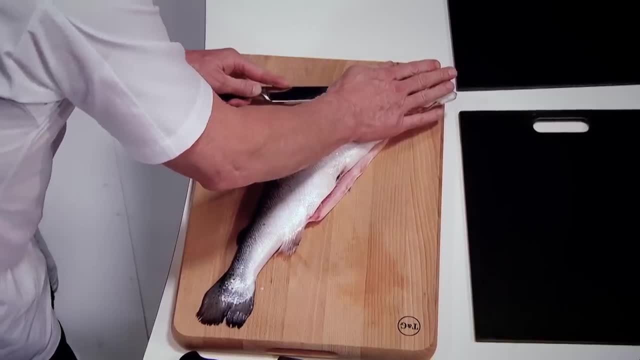 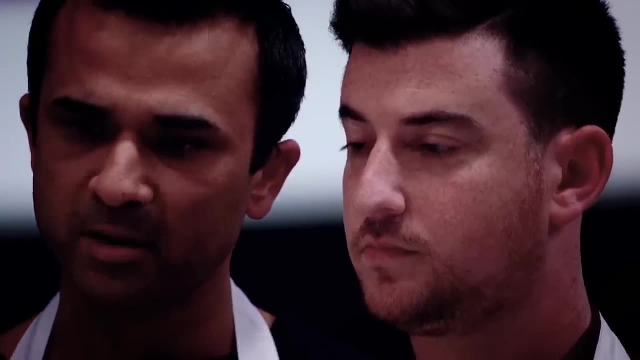 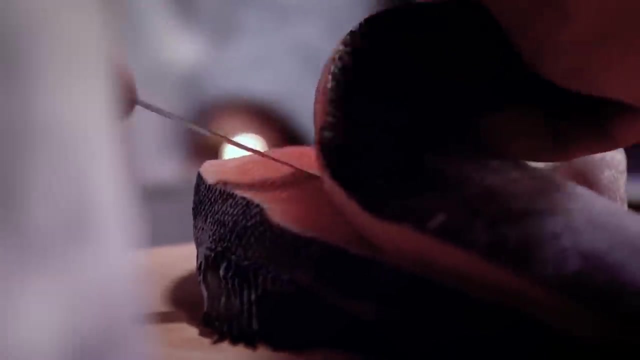 to cut through the salmon. Use your hand, Use the tip of the knife. Hear that noise. That's the rib cage. Come down all the way through. Clean the knife every time. Lift up the salmon, slice through, keeping the knife nice and flat. If it's not flat, you're gonna cut a huge hole in that salmon Now. 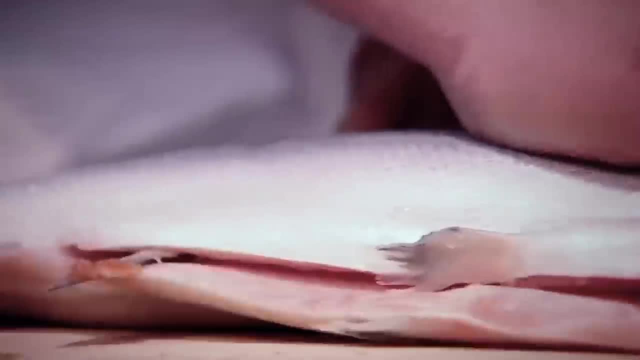 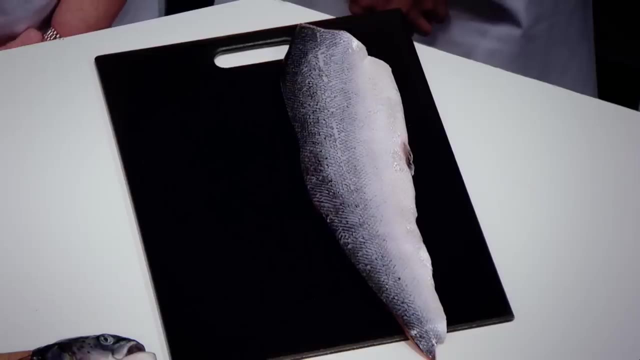 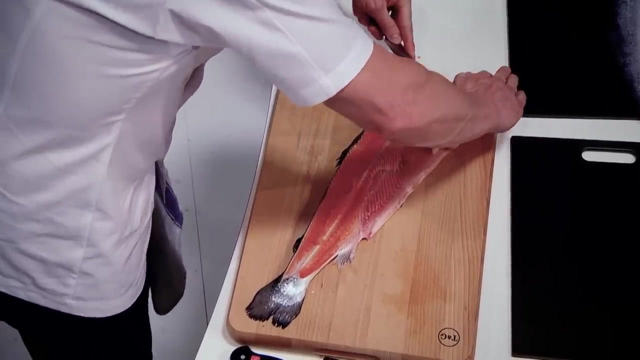 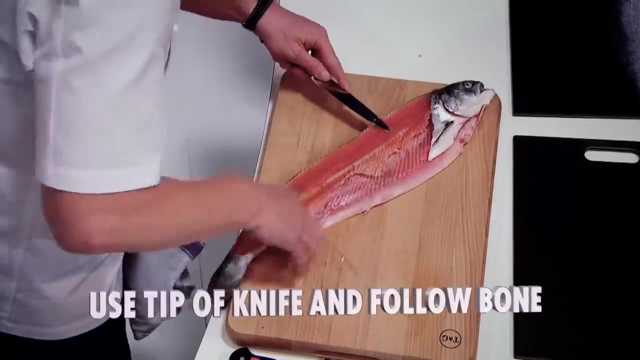 check what you're doing. Place the salmon back down. Let the knife come down. Flip through Clean knife every time It will sharpen. Hold the head nice and firm. Knife down in and through. Be very careful here not to go too deep. I'm using the tip of the knife and literally just coming in. 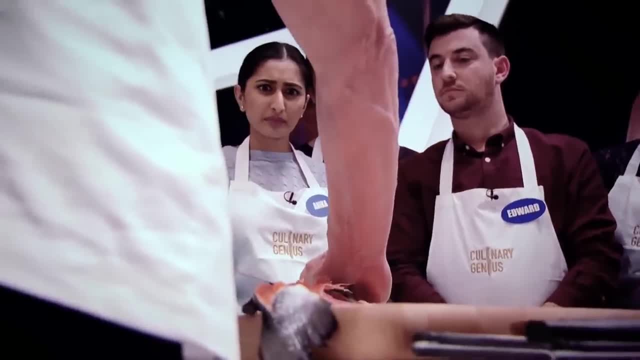 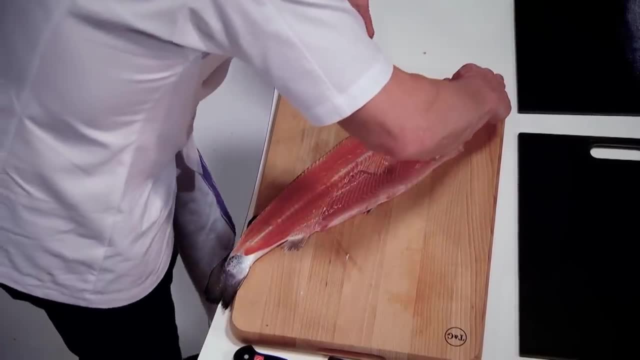 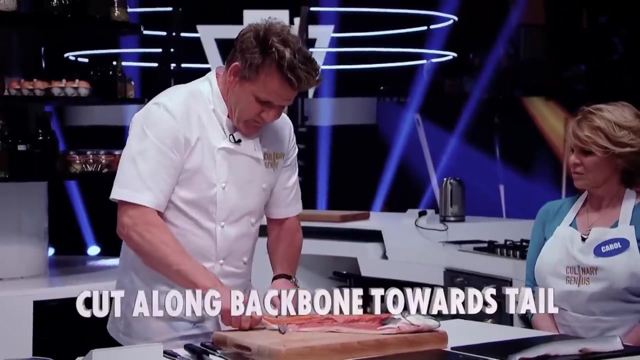 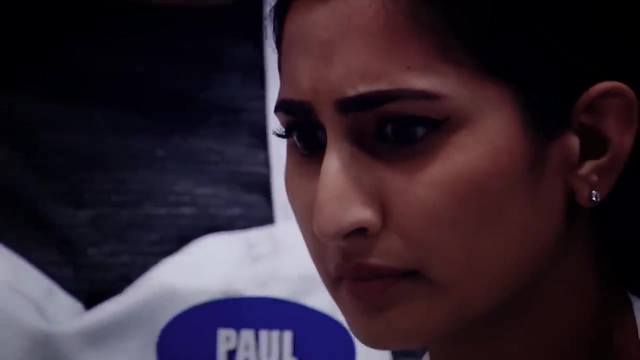 and across that bone. See, Follow that bone down. If the knife gets dirty, pull it out, clean it. come back up. hold the salmon nice and firm Now, let the knife do the work. okay, Through and off Now from there. slice that off, Take that. 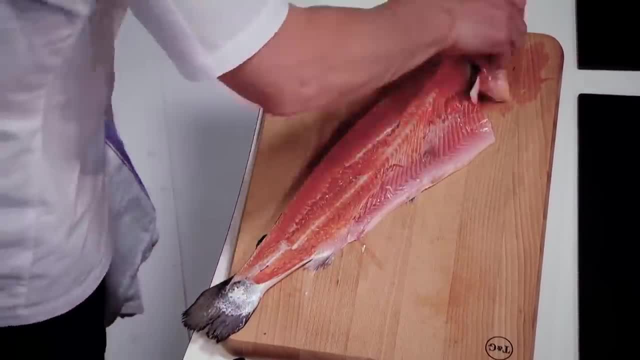 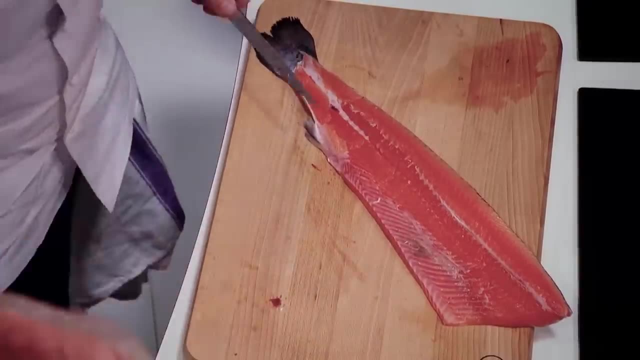 off, lay that back down and come through there. I want to see a nice, clean carcass like that. I don't want to see any salmon left on there. Trim round the salmon and this is where you take these first fine bones out. Don't go too deep. You don't want to go too deep. Don't go too deep.